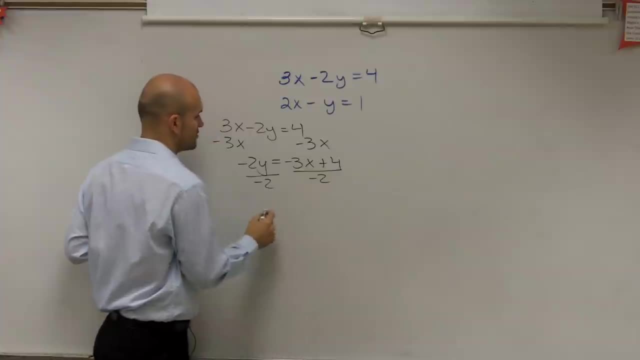 Then I need to divide by the negative 2.. So I have: y equals negative. 3 divided by 2 is a positive. 3 halves x. 4 divided by negative 2 is a minus 2.. Now a lot of you might say, ooh, fraction. I don't like it. 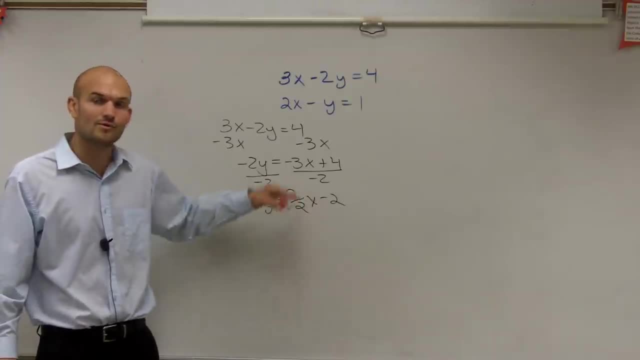 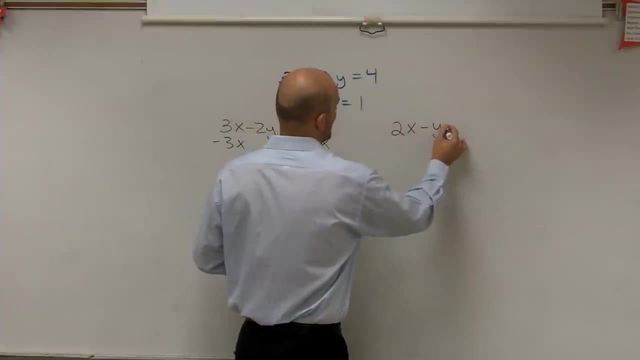 But remember, this is our slope, so this is actually going to be very helpful when we go ahead and try to graph this line. So the next one, let's write: we have 2x minus y equals 1.. Now I'm just going to get the y by itself, right? 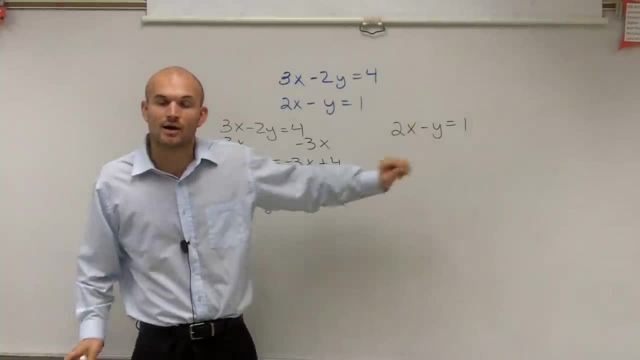 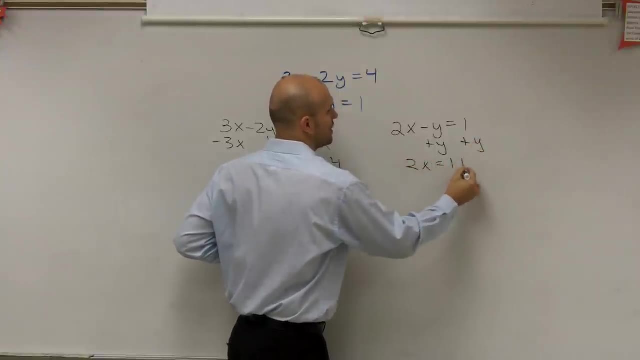 So I could subtract the 2x and then divide by negative 1.. However, for this problem I'm actually going to add the y to the other side. So I have 2x equals 1 plus y, and then I'll just subtract the 1.. 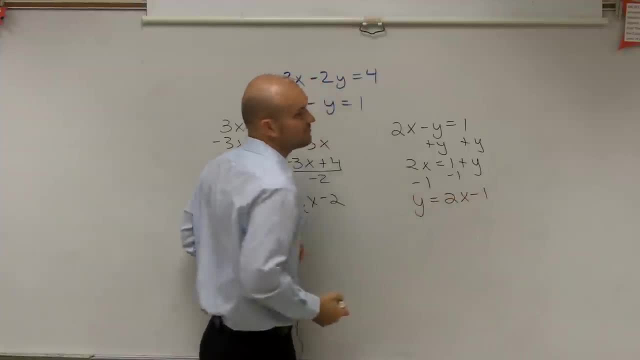 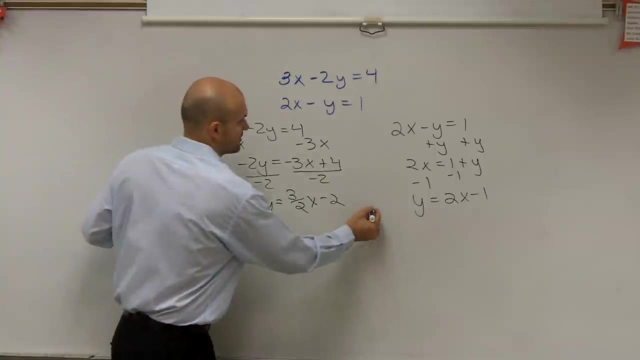 So my final answer is: y equals 2x minus 1.. So now, how do you graph, guys? How do you? How do you? How do you graph these two equations? Well, remember your equations. we're going to set up with an x and a y axis. 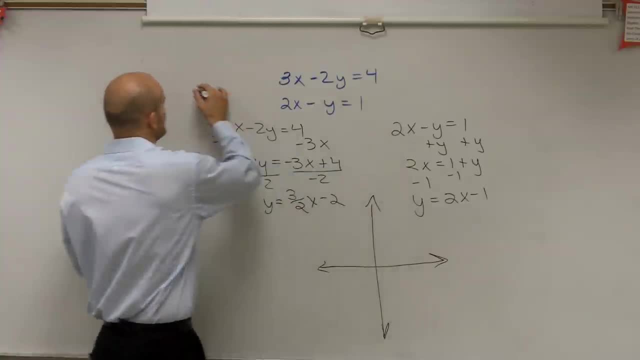 All right. So remember, when it's in y equals mx plus b form, we put it in this form so we could remember a couple things. This is your y intercept, right? And it's your y intercept at 0 comma b. 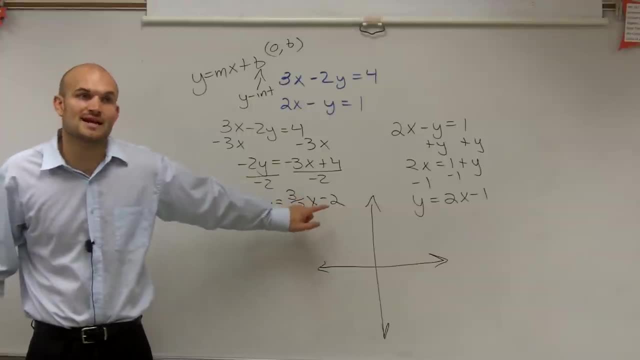 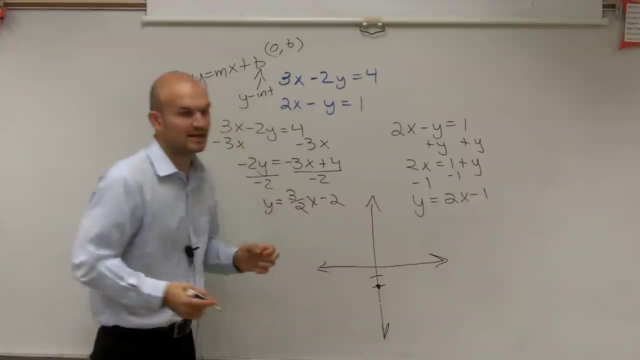 So I'm going to go down. So I look at here and I say my y intercept's at negative 2.. That means this graph, This graph crosses at negative 2.. So I go down to negative 2, and I make a nice little dot. 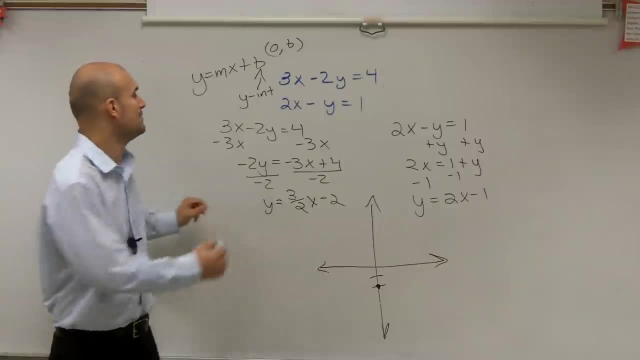 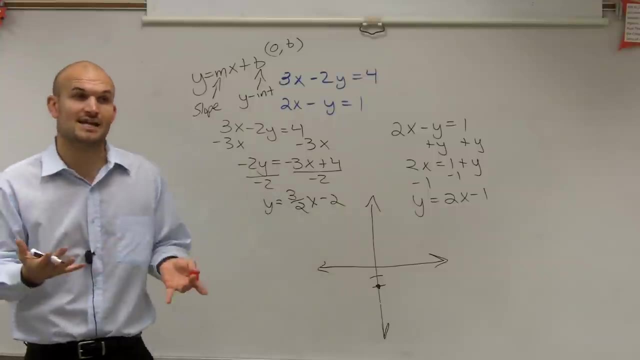 Then it says my slope is going to be 3 over 2.. And remember, because your m is your slope, remember slope we represent like as a rise over 1. It's the change in your y values over the change in your x values. 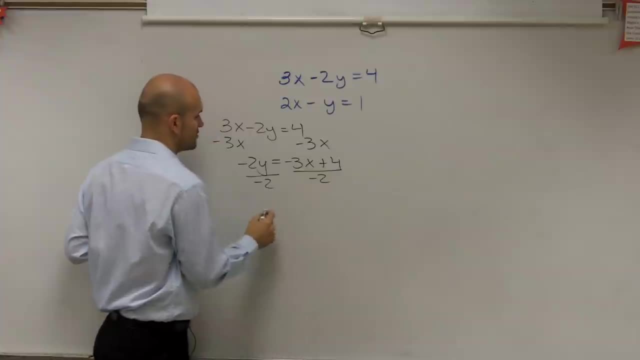 Then I need to divide by the negative 2.. So I have: y equals negative. 3 divided by 2 is a positive. 3 halves x. 4 divided by negative 2 is a minus 2.. Now a lot of you might say, ooh, fraction. I don't like it. 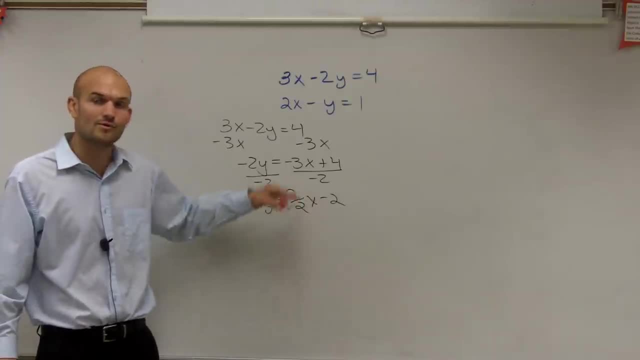 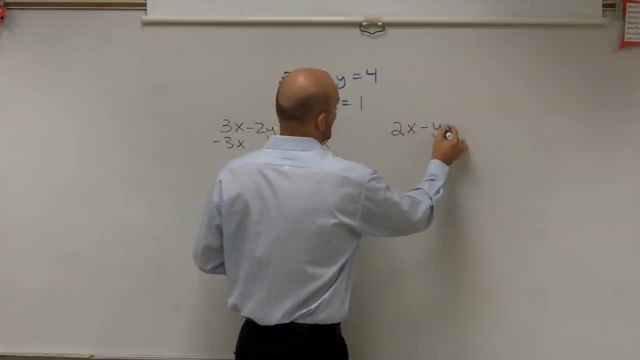 But remember, this is our slope, so this is actually going to be very helpful when we go ahead and try to graph this line. So the next one, let's write: we have 2x minus y equals 1.. Now I'm just going to get the y by itself, right? 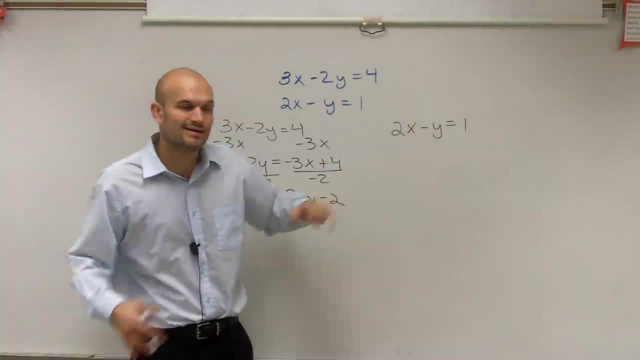 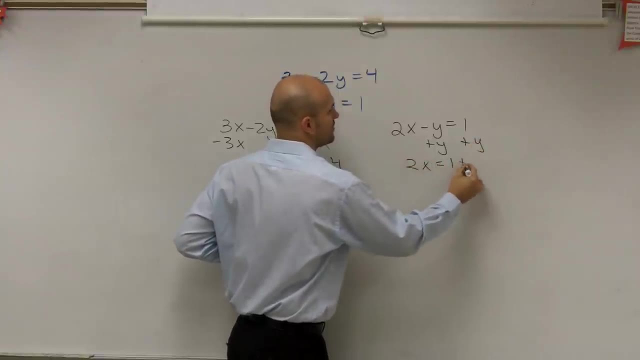 So I could subtract the 2x and then divide by negative 1.. However, for this problem I'm actually going to add the y to the other side. So I have 2x equals 1 plus y, and then I'll just subtract the 1.. 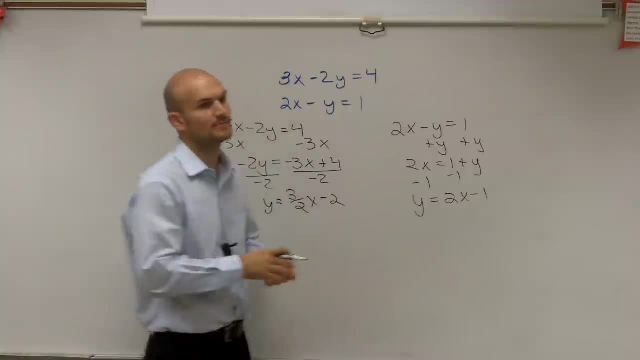 So my final answer is: y equals 2x minus 1.. So now, how do you graph, guys? How do you graph? How do you graph these two equations? Well, remember your equations. we're going to set up with an x and a y axis. 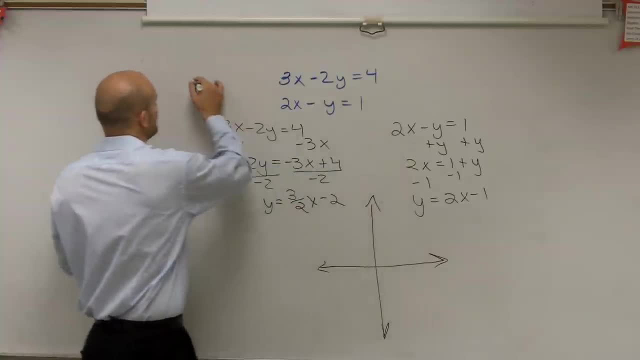 All right. So remember, when it's in y equals mx plus b form, we put it in this form so we could remember a couple things. This is your y-intercept, right? And it's your y-intercept at 0 comma b. 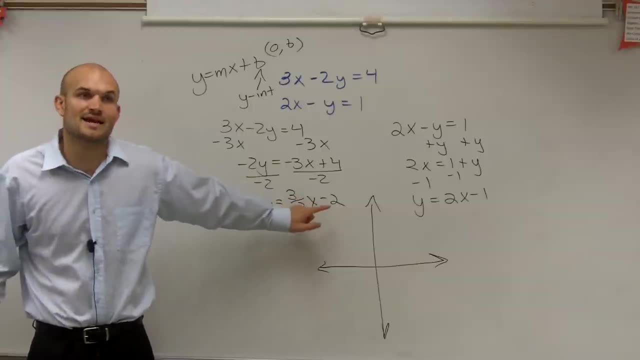 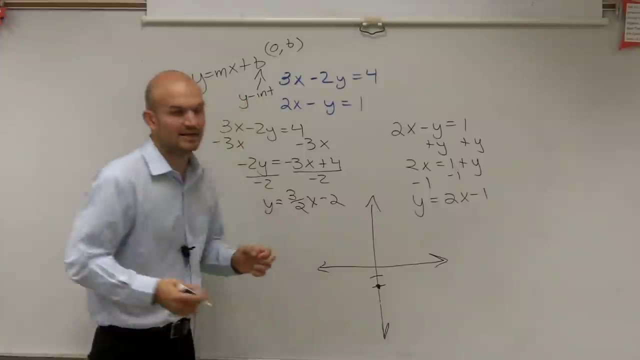 So I'm going to go down. So I look at here and I say my y-intercept's at negative 2.. That means this graph crosses At negative 2.. So I go down to negative 2, and I make a nice little dot. 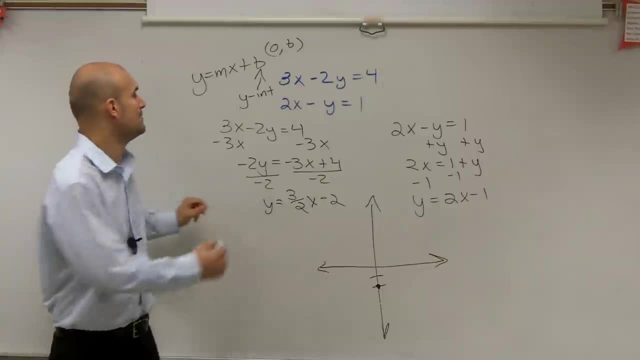 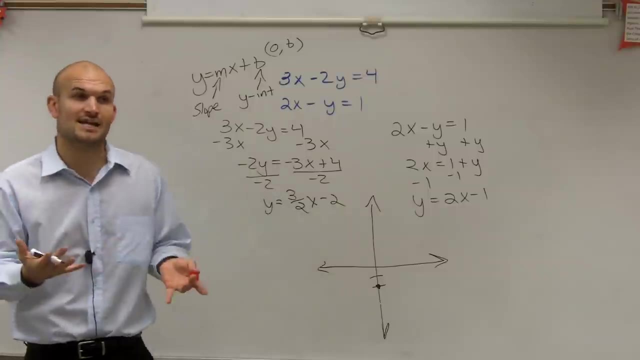 Then it says my slope is going to be 3 over 2.. And remember, because your m is your slope, remember slope we represent like as a rise over 1. It's the change in your y values over the change in your x values. 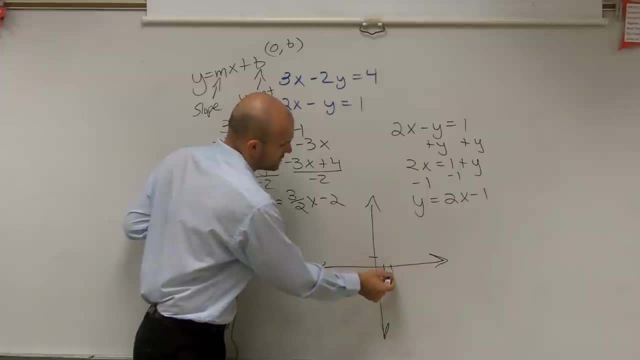 So I'm going to go up 3, 1, 2, 3, over 2.. So that's going to take me to my next point. You could also do a negative over negative, because that would still be positive. 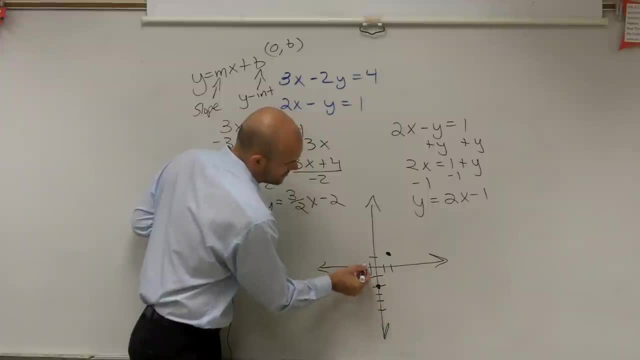 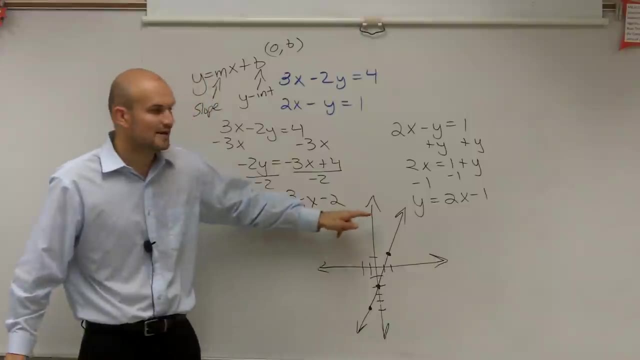 You could also go down 3,, 1,, 2,, 3, to the left, 2.. And then I connect my two point, or connect my points, and I have my line. Make sure, ladies and gentlemen, I've seen a lot. 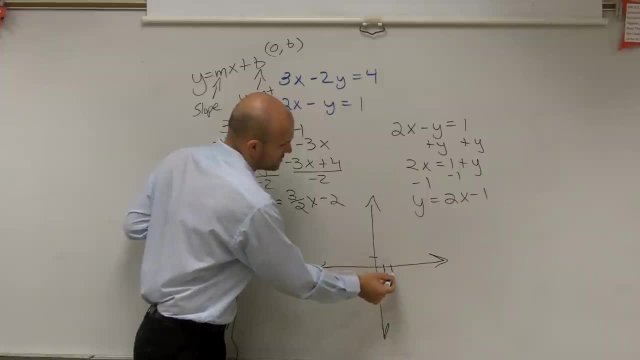 So I'm going to go up 3.. 1, 2, 3 over 2.. So that's going to take me to my next point. You could also do a negative Negative over negative, because that would still be positive. 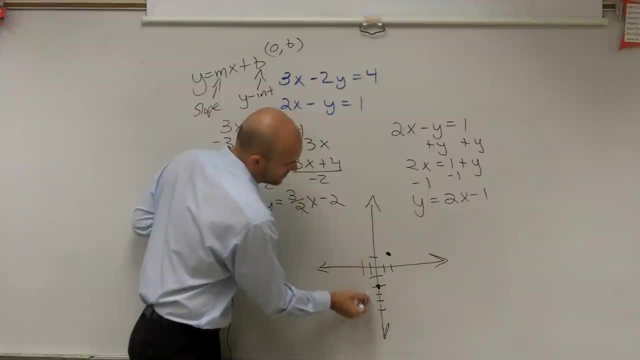 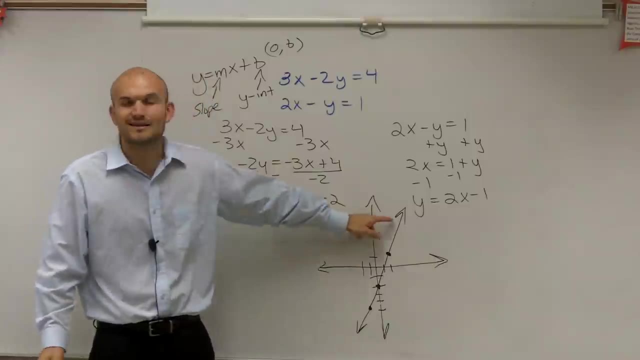 You could also go down: 3.. 1,, 2,, 3 to the left: 2.. And then I connect my two point, or connect my points, and I have my line. Make sure, ladies and gentlemen, I've seen a lot of people graphing and they're not putting the arrows right. 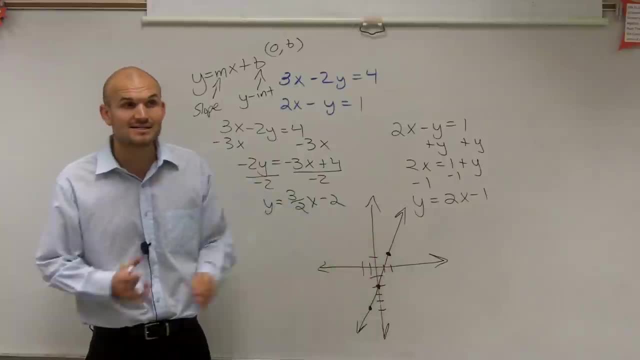 of people graphing and they're not putting the arrows right. When we're graphing lines, they have infinite length, So make sure you create those arrows at the end. The next one: it says 2x minus 1.. 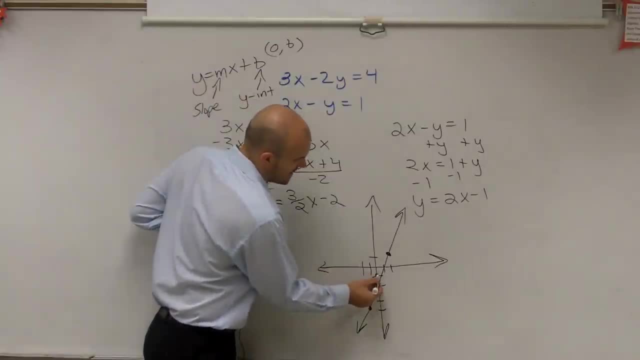 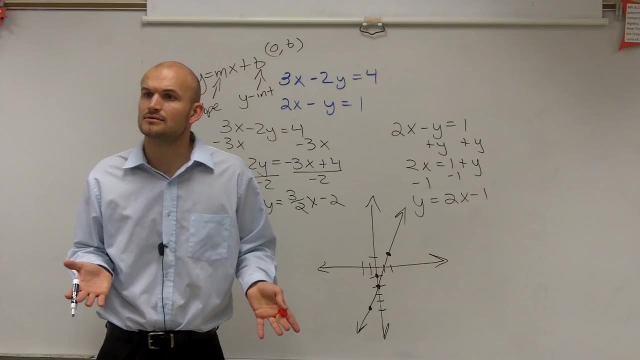 So now this one goes down at negative 1, right So, but my slope is a 2.. Well, how do you do change in y over change of x? It's going to be your chain. you need to make sure. 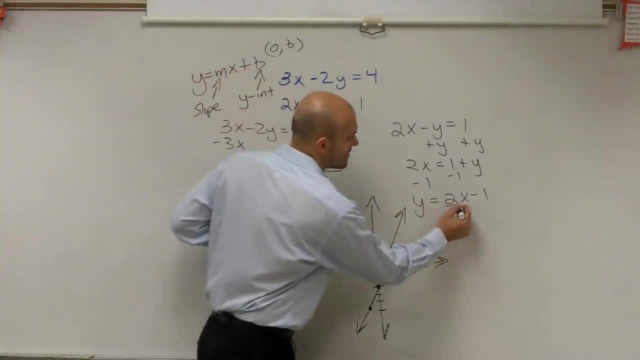 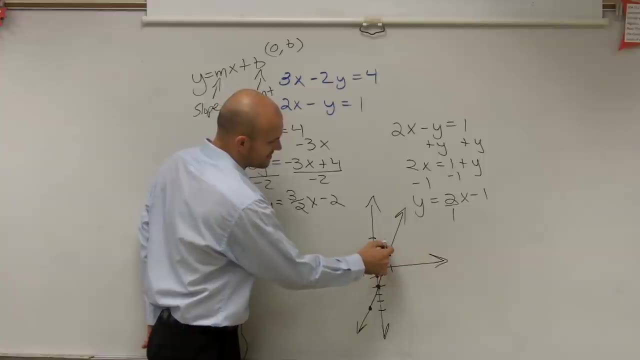 you have to write this as a fraction. So actually, we're going to want to make sure we write as a fraction with 2 over 1.. So, therefore, I'm going to go up 2 over 1. And if I keep going like that, 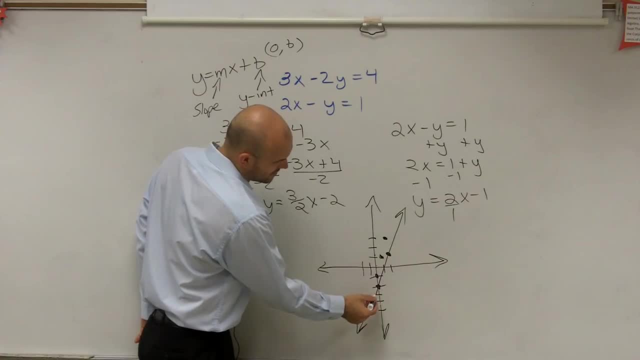 I notice that these aren't going to graph. However, if I go down 2 to the left one, we notice that they- if my graphs are a little bit okay, but we notice that they intersect at a certain point. So what was that point?